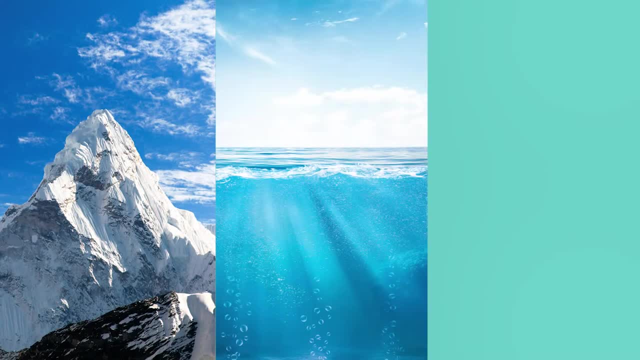 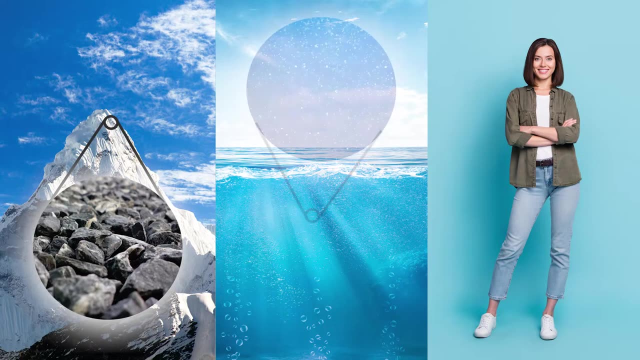 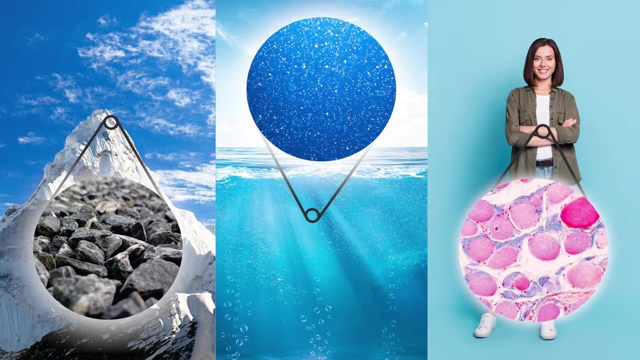 What do Mount Everest, the Atlantic Ocean and the human body have in common? The rocks and soil that make up mountains, the complex mixture of water, salts and gases that compose our oceans and the microscopic cells that form our bodies are all made of. you guessed it. 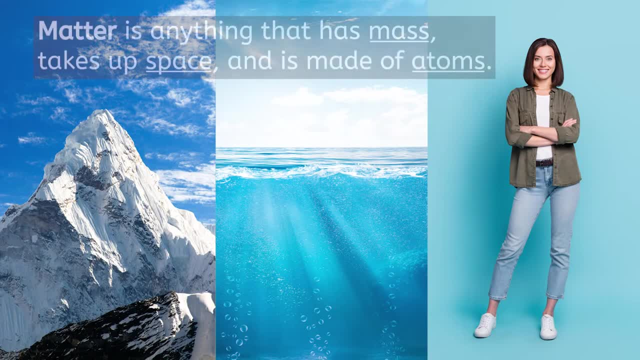 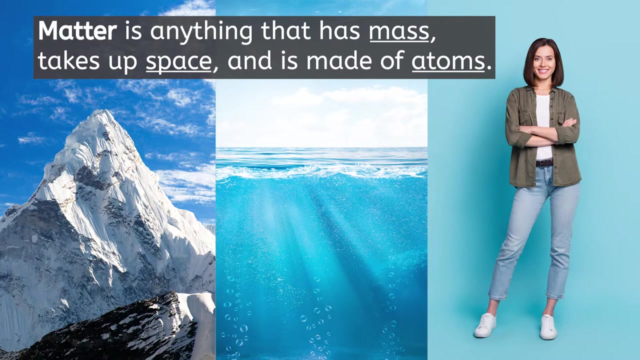 matter. According to Merriam-Webster, matter is anything that has mass, takes up space and is made of atoms. Well, that sounds like pretty much everything right, But what exactly is matter? And how can a mountain, the ocean and you and I all be made of the same things? 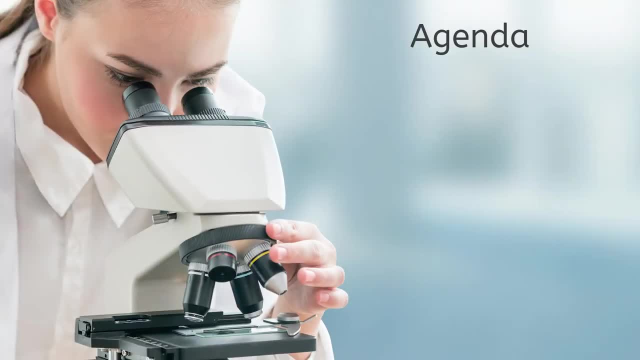 We're going to find out. By the end of this lesson, you'll be able to define what matter is and where it can be found. You'll also be able to describe the properties of the solid, liquid and gaseous states of matter. Get ready, because we're about to explore some. 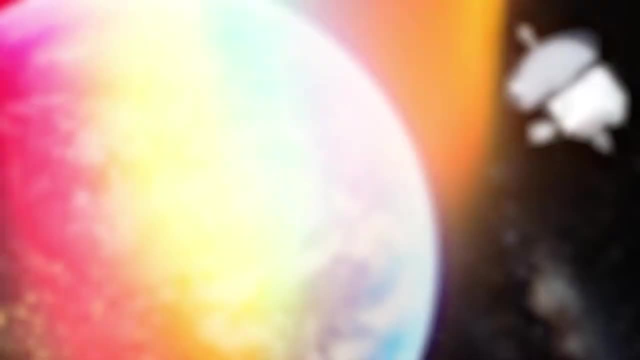 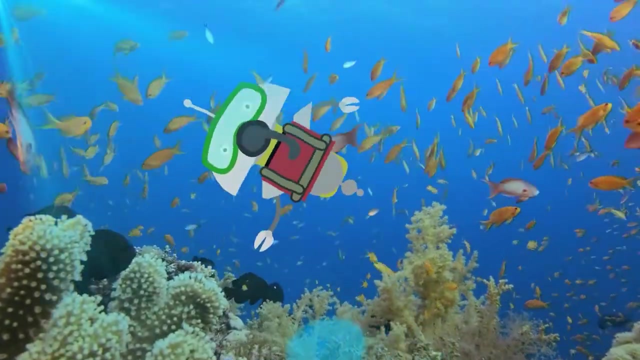 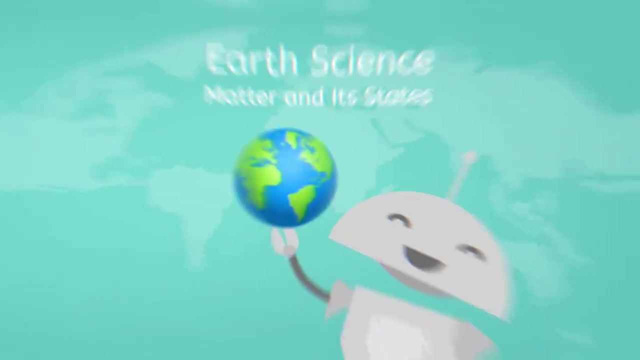 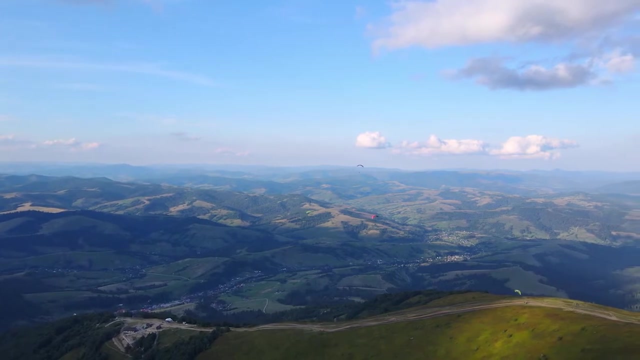 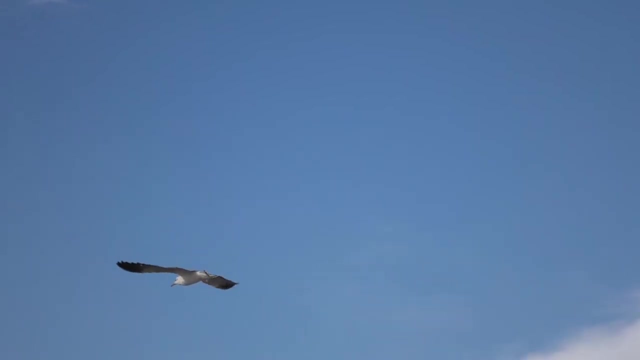 really tiny science. Matter is everywhere. Even the air we breathe is matter. There are really only a few things that aren't matter, like light, heat and sounds. We can't hold taste or smell these things because they aren't matter Instead. 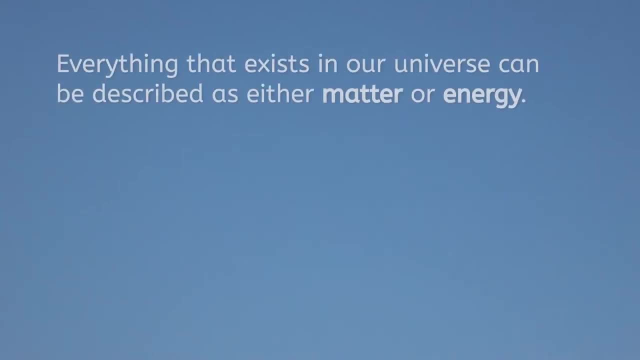 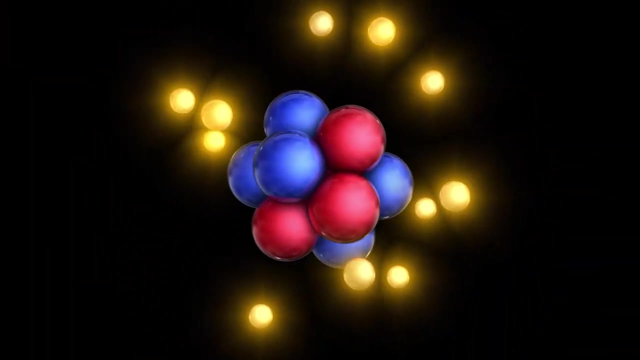 they are types of energy. In fact, everything that exists in our universe can be described as either matter or energy. So let's take a closer look at matter. All matter is made of atoms. You can think about atoms as the tiniest building blocks that all the matter. 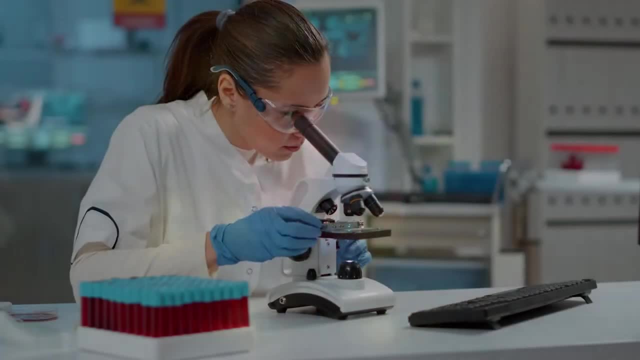 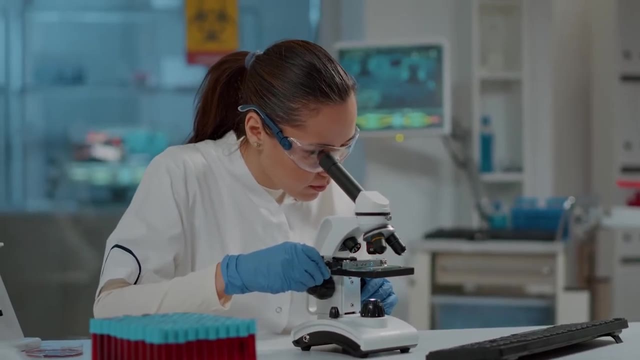 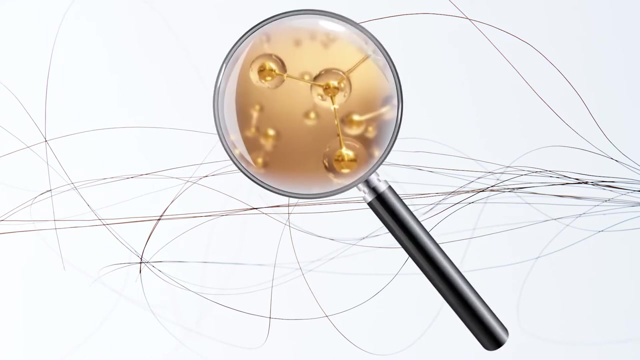 around us is made of. Atoms are far too small to see with our eyes. Only the most powerful microscopes can allow scientists to observe them. Think about the width of a single strand of hair. Each hair is about a million atoms wide. They are seriously tiny. 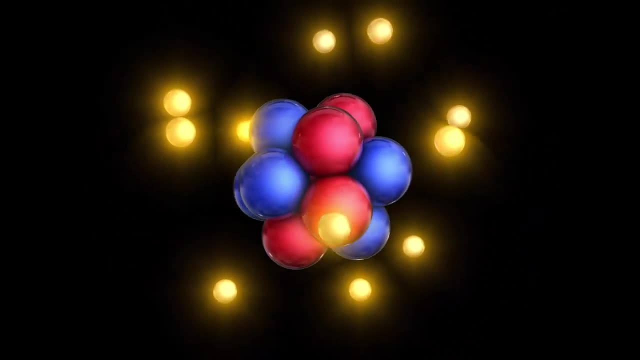 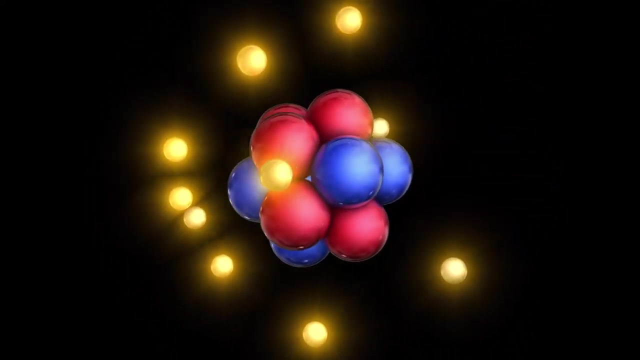 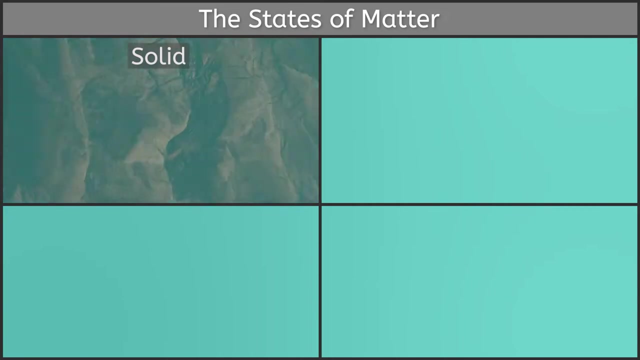 Now, all matter is made of atoms. How these atoms behave is what makes rocks, water and the air around us all different Scientists categorize matter into four groups, which are called the 4 states of matter: Solid, liquid gas and plasma …. However, in this lesson, 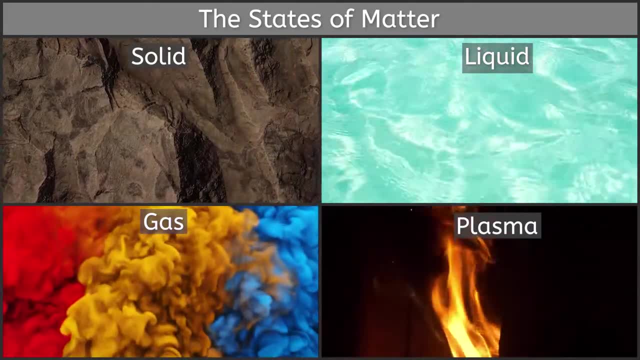 we'll focus on the first three because on earth, matter in the Plasma state isn't very common. Let's take a look at remaining tet 1973.. Let's start by taking a look at what fertilizers do We have carbon dioxide, phosphorus, ammonium, tilhyde, potassium and sulfur, and you'll be the first to see. that The top, Which I'd always mean, compared to natural puesetia. attention with, however, in this lesson. That's how matterCRIES to matter, though homeless on Earth, Whoret, and you've gotten to know us on our minds about this. 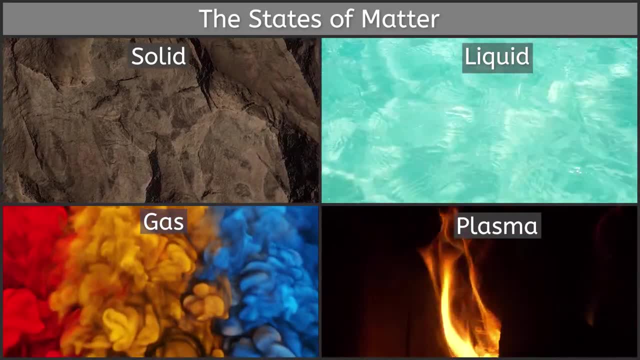 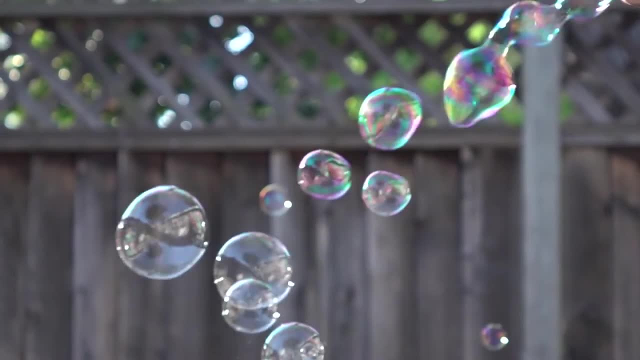 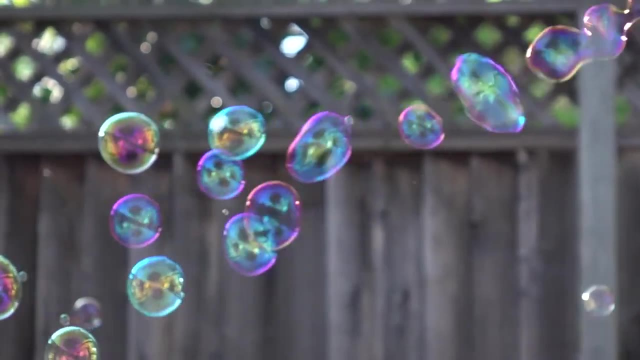 the state of matter that's all around us all the timegas. It's probably easy to spot some solids and liquids around you right now, but can you see any gases? Most of the time, we can't actually see gases in the world around us, even though 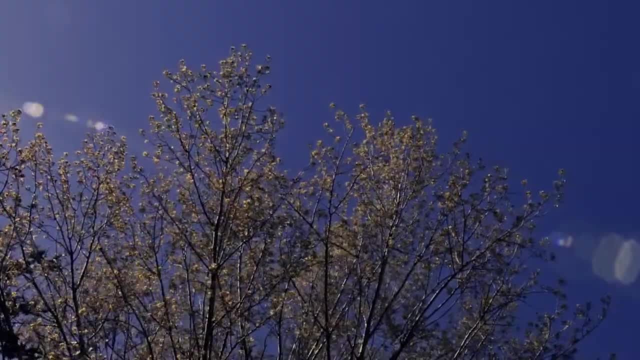 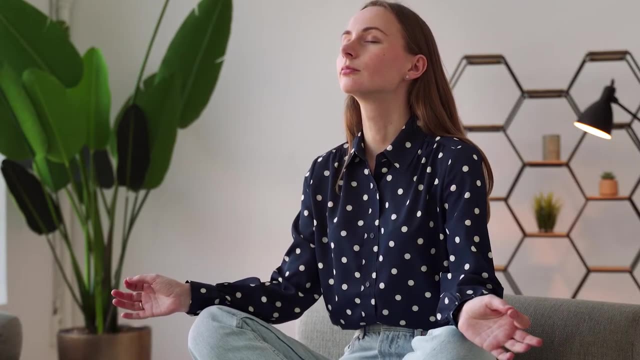 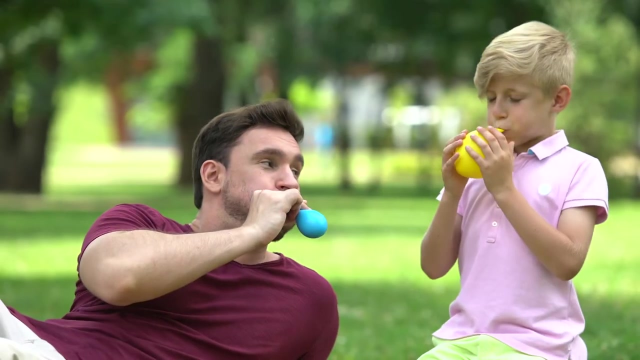 they really are everywhere. Gases are in the air, in the carbonated drinks we enjoy and even in our bodies. So you might be wondering: if we can't always see gases, how do we know they're really there? Well, imagine blowing up a balloon. 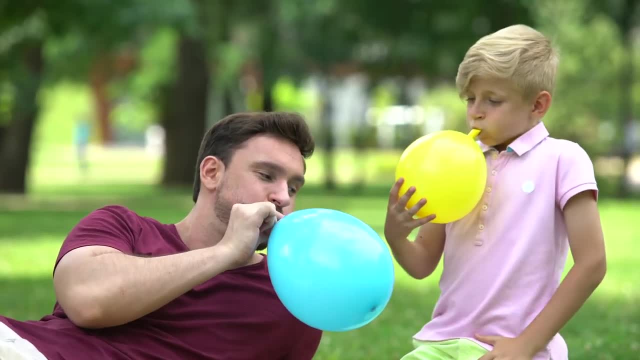 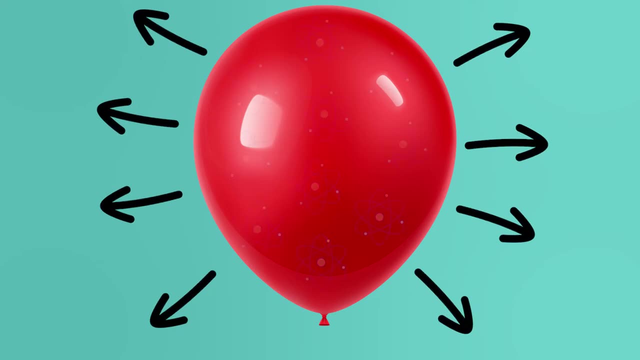 As you blow in more and more air, the balloon gets bigger and bigger. This proves that gas takes up space, since it can push out the sides of a balloon. But what are the atoms in a gas doing that makes them so different from other states? 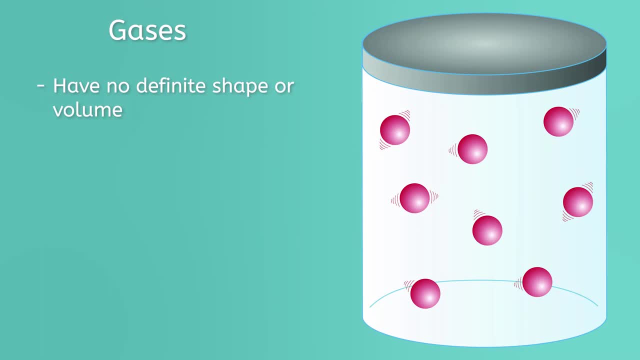 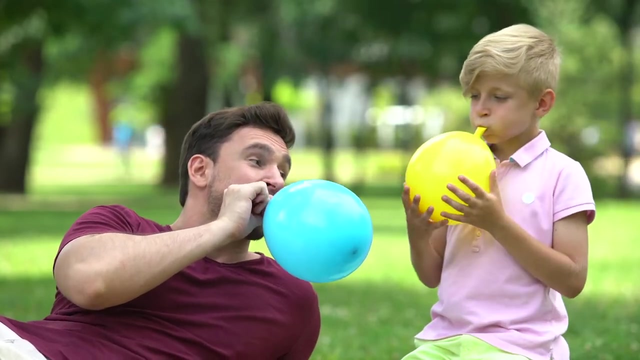 of matter. Gases don't have a definite shape or volume, which is the amount of space an object takes up. Gases actually spread out to take up whatever space is available to them, For example, gases such as the air inside a balloon spread out so that the space inside 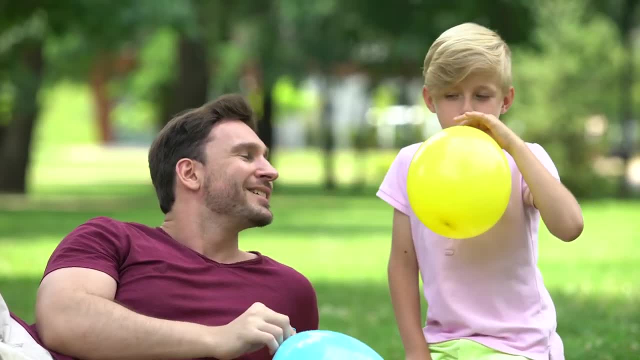 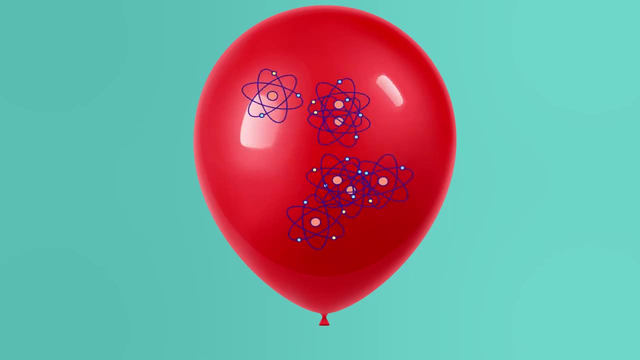 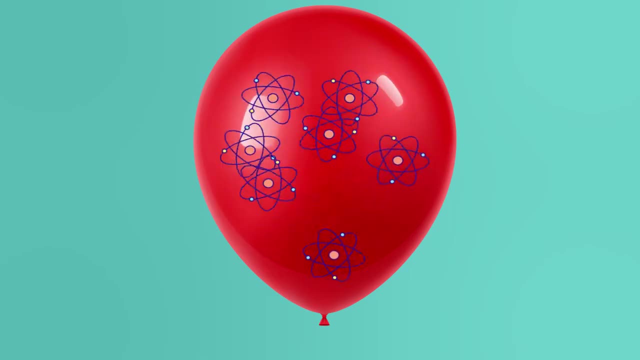 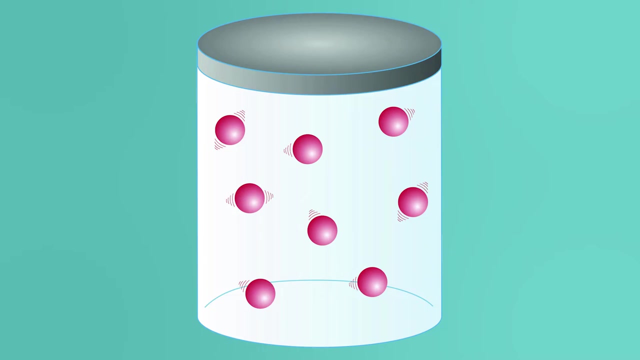 They're constantly moving. They're constantly moving. They're constantly moving. They're constantly jumping around and bumping into each other and they'll keep going until they hit the sides of the container they're in. So gas atoms move very quickly and are spread pretty far apart. 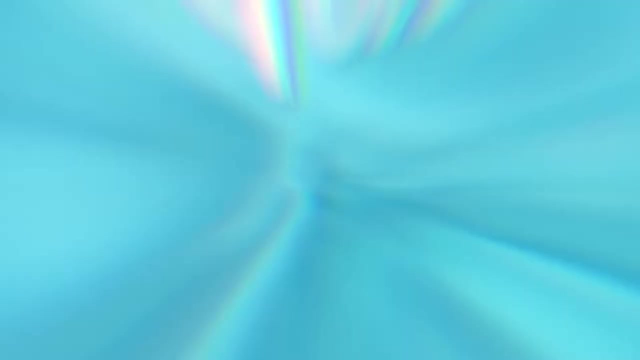 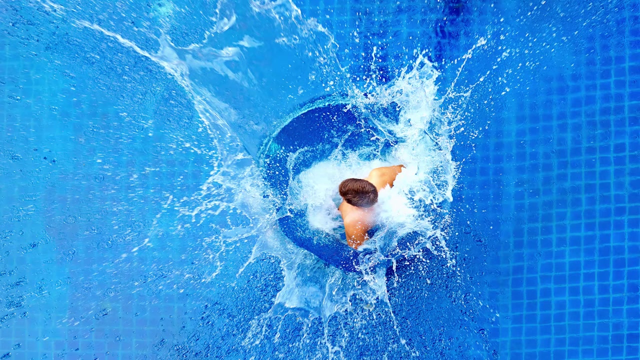 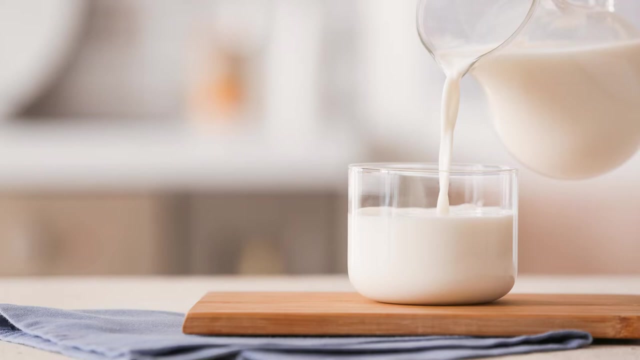 But this isn't the case for every state of matter. We owe the refreshing experience of swimming in a pool, the warm deliciousness of maple syrup and the creamy goodness of fresh milk to our second episode of this series. The second state of matter: liquids. 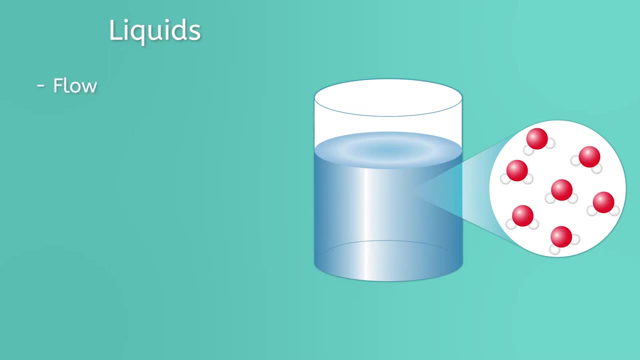 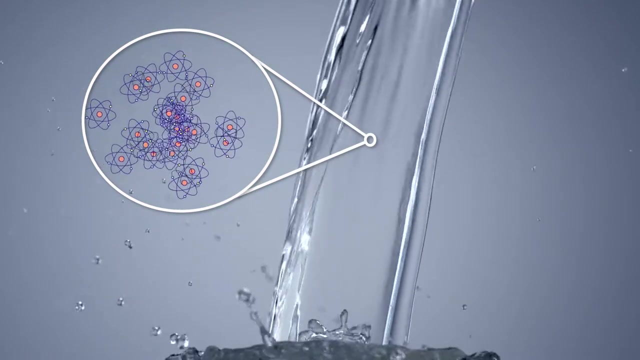 Some important characteristics of liquids are that they flow and, while they have a definite volume, they don't have a definite shape. So, like gases, they take the shape of whatever container they are poured into. This happens because atoms in a liquid are closer together than in a gas, but they still 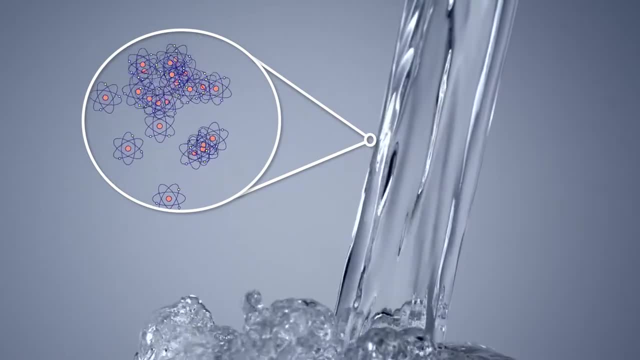 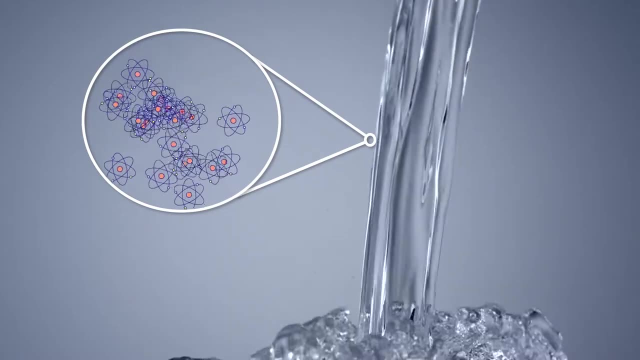 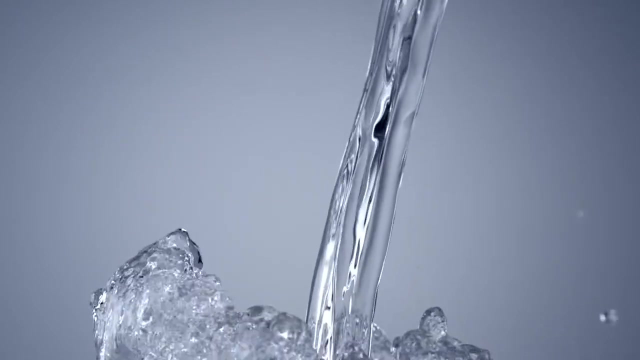 don't have a clear arrangement. As a result, they're able to quickly move. They can easily move past each other. As they do, so, other atoms in the liquid slide in to fill the empty spaces. This is what makes liquids flow when we pour them, which is way different than our next. 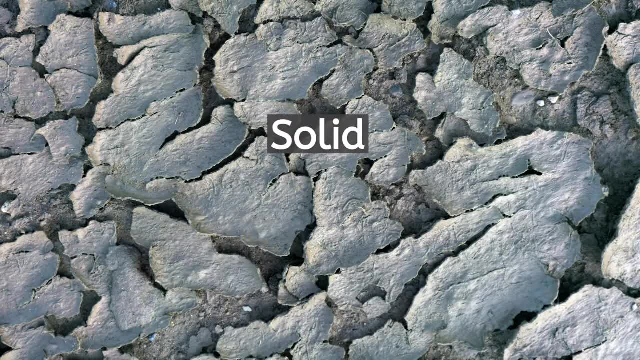 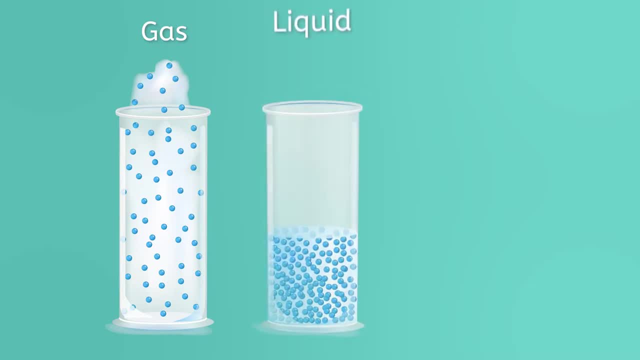 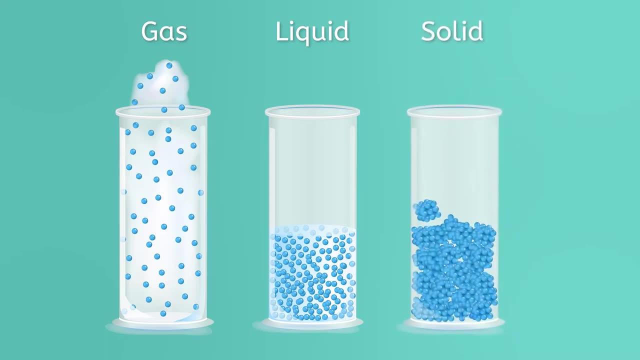 state of matter. We know that in gases there's lots of space between atoms. In liquids the atoms are closer together but still free to move around. But solids are a bit different. Take a look at the atoms in this solid grain of salt. 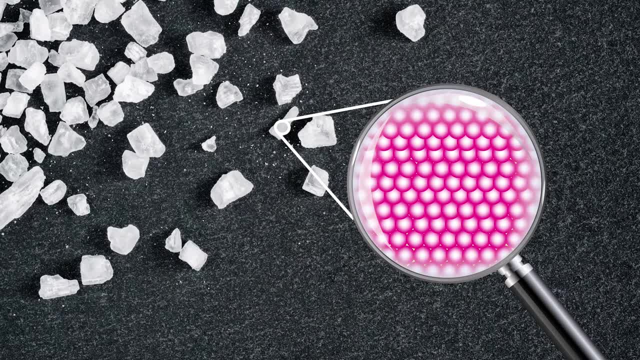 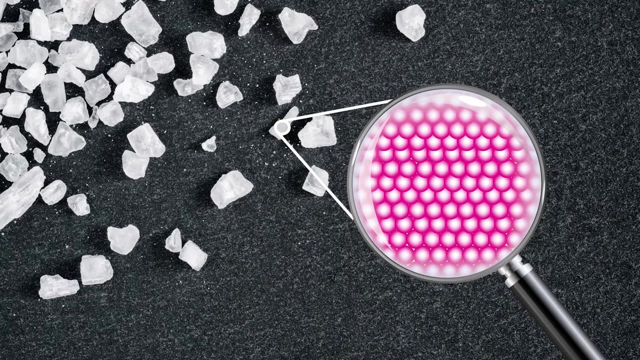 Now that you know some of the important characteristics of gases and liquids, what do you observe about this solid Think about ways that the atoms you see here are both similar to and different from what we've already seen in gases and liquids. Then pause the video here to fill in your observations. 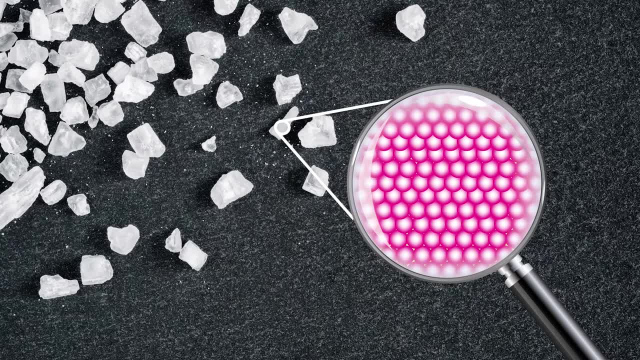 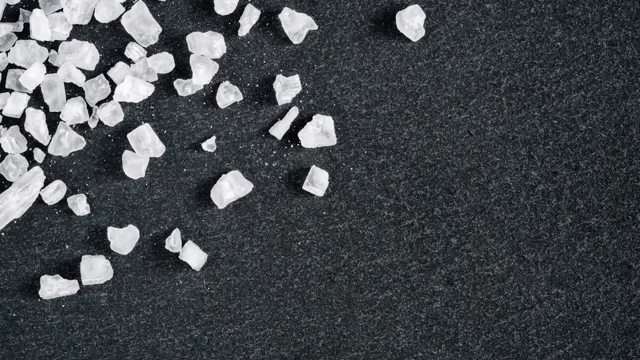 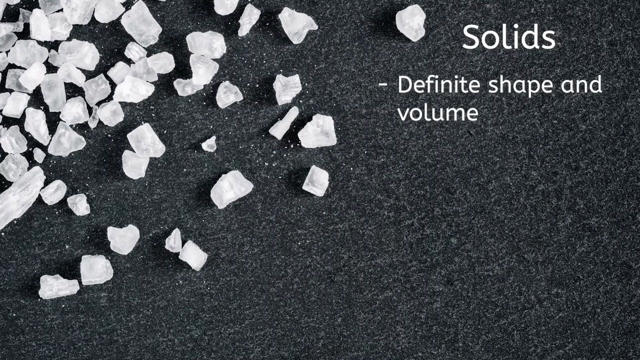 See you next time. Well, what did you observe? In solids, the atoms are packed together really tightly. There's just about no space between them. That's why, unlike gases and liquids, solids have a definite shape and volume, like a wooden. 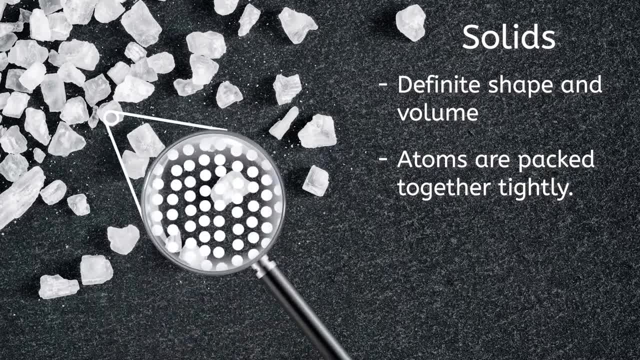 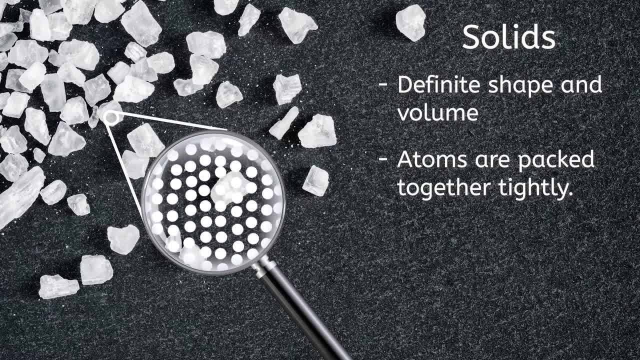 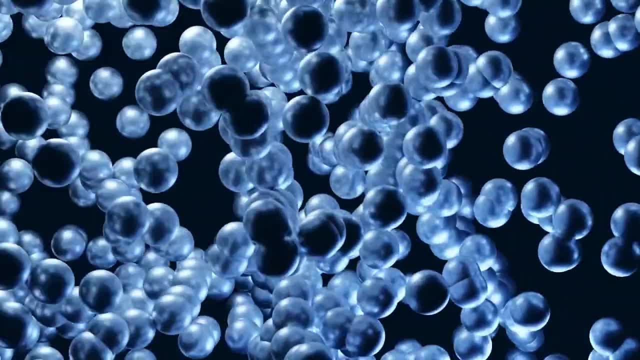 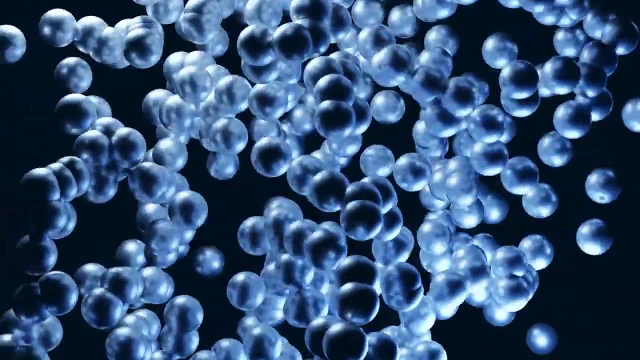 They just don't move as much as the atoms in a gas or a liquid. Instead, they basically vibrate while staying in place. These atomic movements, whether large or small, happen because all matter also has some energy within it. The more energy the matter has, the faster the atoms move, which is why gases have more. 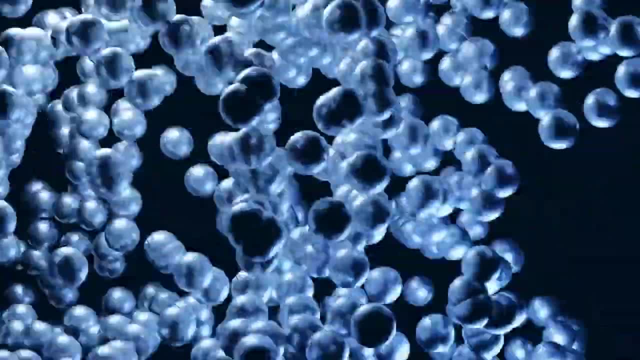 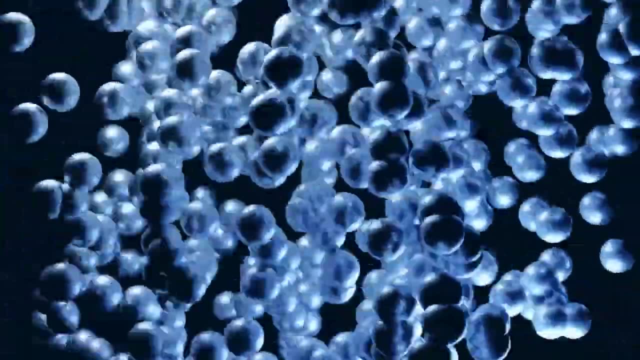 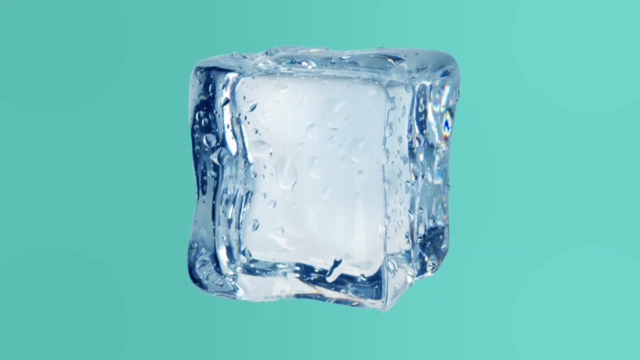 energy than liquids, and liquids have more energy than gas energy than solids. Additionally, changing this level of energy can cause an object to change between the different states of matter. This process is called a phase change. For example, let's take a look at this ice cube. What state of matter do you think it is And what does that mean? 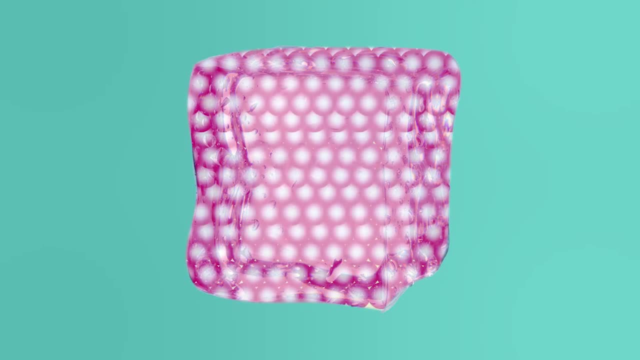 about the energy within it. This ice cube is a solid and that means its atoms don't have too much energy, so they're just vibrating in place. However, what would happen to those atoms if we apply heat energy to this ice cube? Pause the video here and draw your prediction in the space. 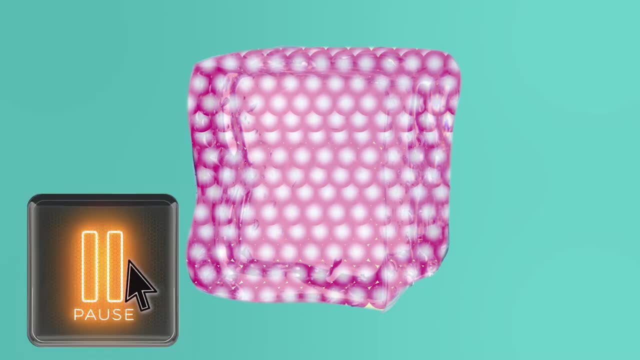 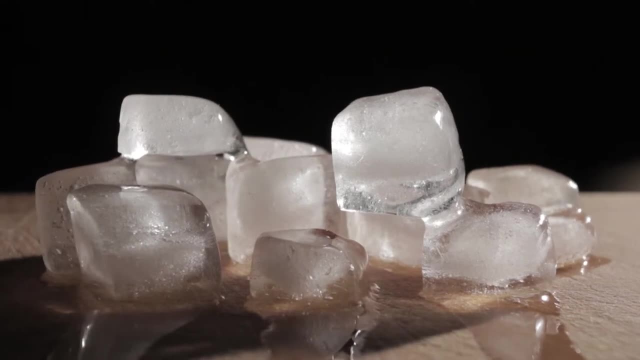 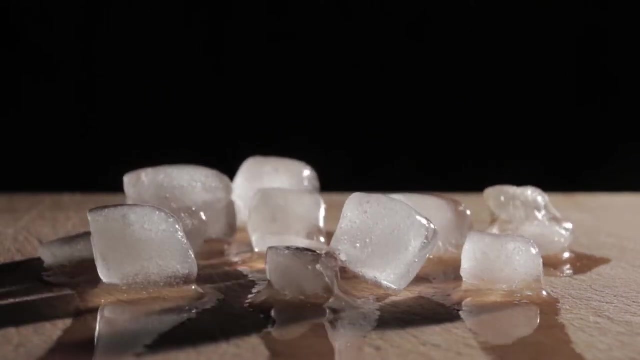 on your guided notes. Applying more energy to these atoms will make them move faster. When they get moving fast enough, they'll even start to flow past each other. And is that change starting to sound familiar If a solid like an ice cube? 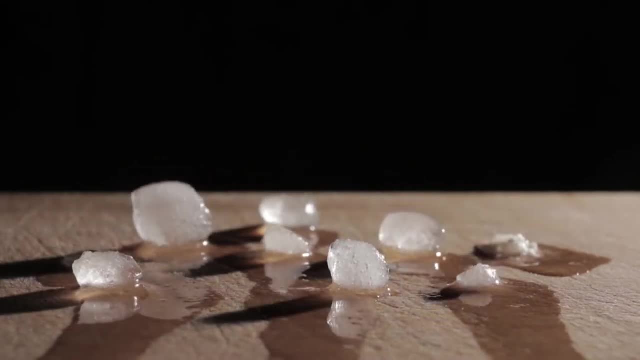 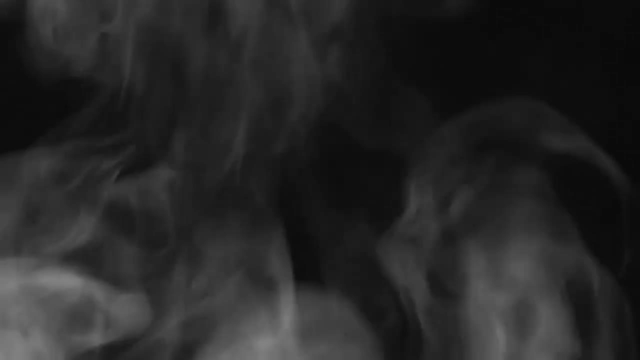 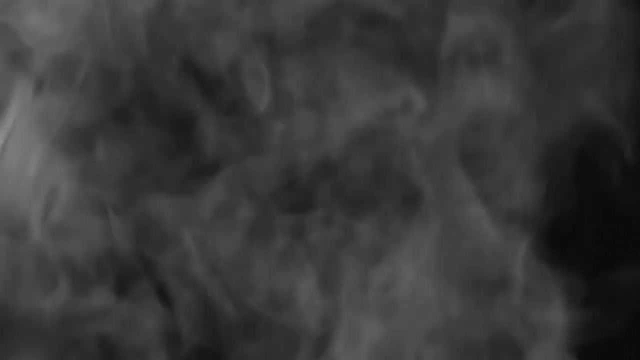 gains enough energy, it can melt into a liquid. In fact, if we keep applying heat, the atoms will continue to gain energy until they're moving fast enough to become a gas. This is why we see water vapor escaping over a pot of boiling water. 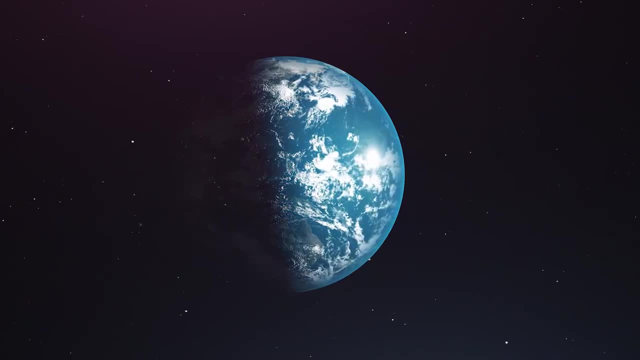 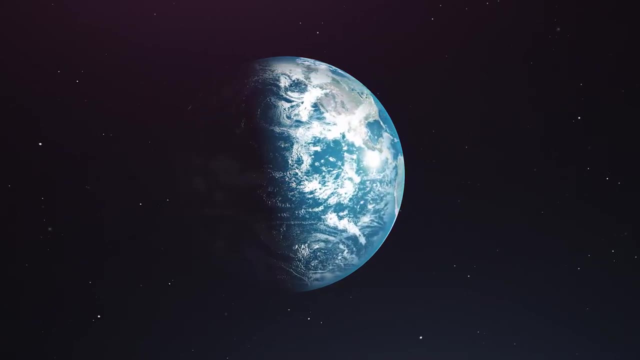 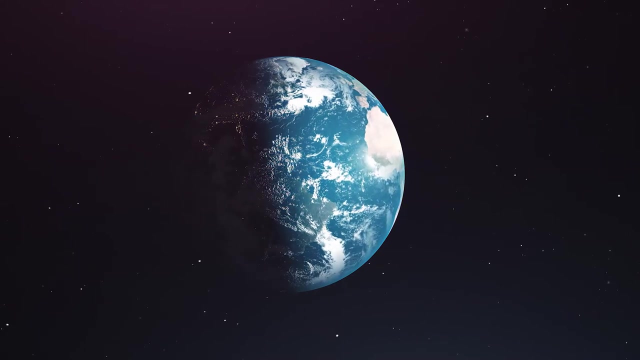 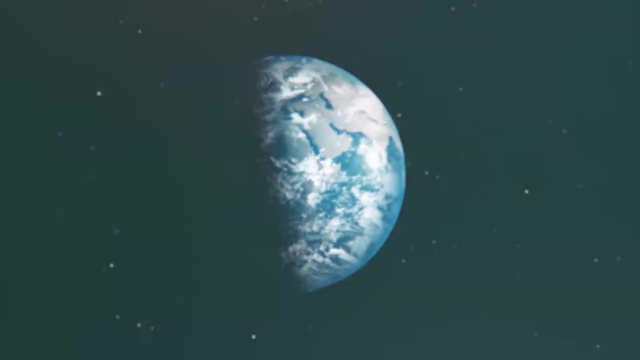 Now you might be wondering: why does matter really relate to earth science? Remember, everything in the universe is either matter or energy. That means every single branch of science involves studying the complex dynamics between these two things, including earth science. The properties of matter help us understand how the tallest 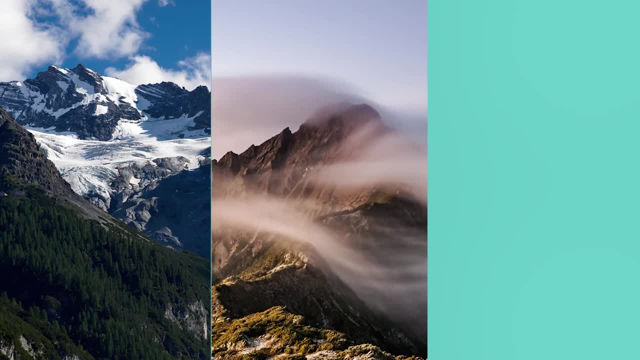 mountain ranges came to be, how weather shapes the face of the earth and even how water circumnavigates the earth. The properties of matter help us understand how the tallest mountain ranges came to be, how weather shapes the face of the earth and even how water circumnavigates the earth.